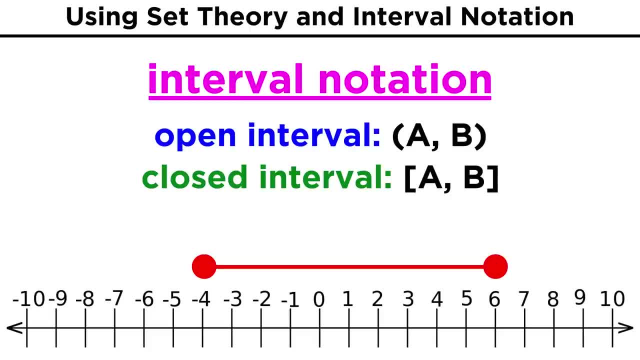 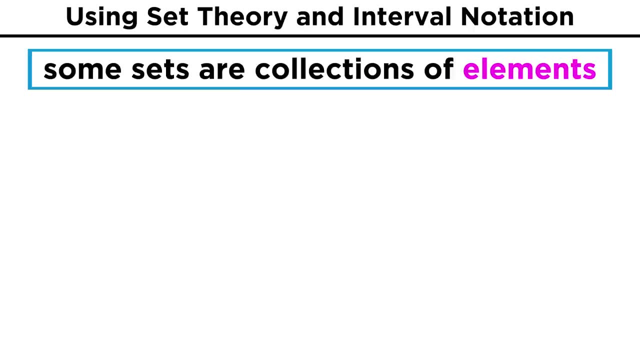 and B and including A and B themselves. Sets that include positive or negative infinity are called infinite intervals. We can also have sets that are not continuous intervals but rather just collections of elements. These utilize this other type of bracket and they just list all of the elements that 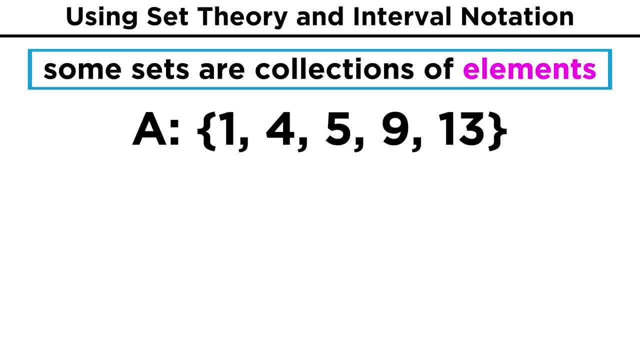 are included in the set, separated by commas. We could have a set like this which includes the numbers one, four, five, nine and thirteen. Then let's say, we have a set like this which includes the numbers one, four, five, nine. 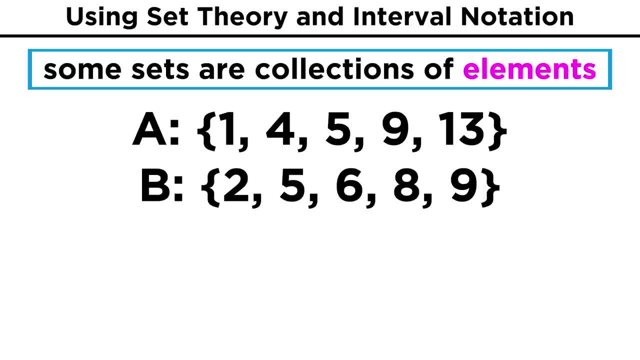 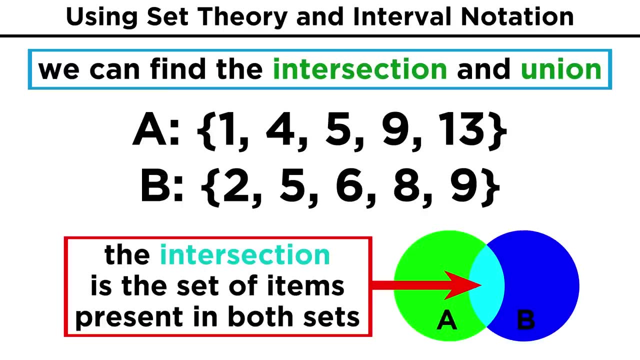 and thirteen. Then let's say, we have another set like this, which includes two, five, six, eight and nine. One thing we could do would be to describe the intersection and the union between these two sets. The intersection of two sets includes all the items that are common to both sets. 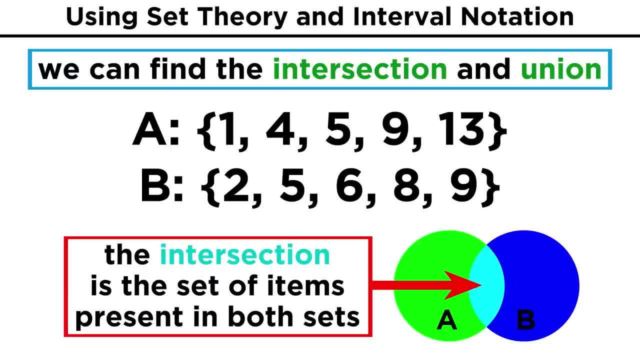 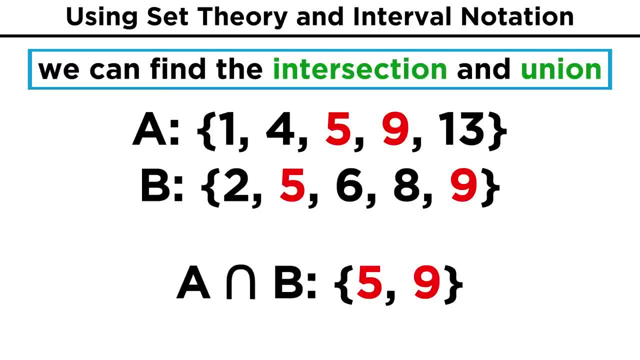 We can think of this as the part of a Venn diagram, where the two objects overlap. In this case, the items that are present in both sets are five and nine, so the intersection of these two sets, which we represent with this symbol. that looks like an upside down. 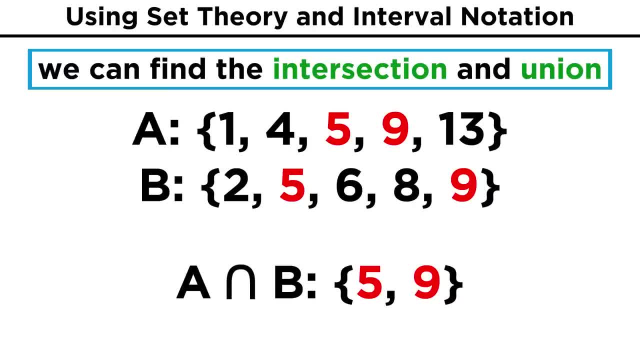 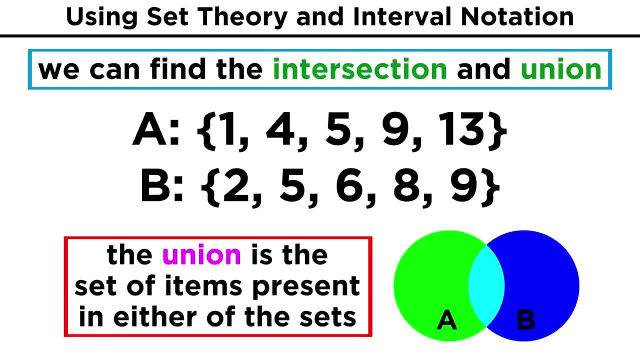 capital U will be the set containing five and nine. By contrast, the union of two sets is the merging of the sets. Every item that shows up in either set will be in the union of the sets. so with the Venn diagram the union is just the whole thing. 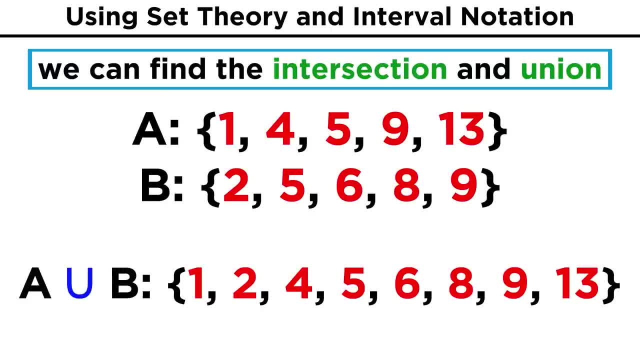 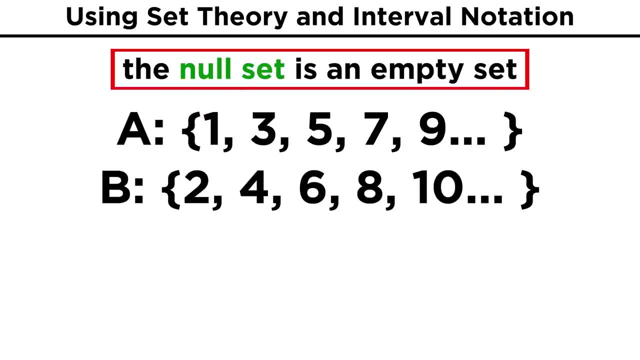 In this case, the union of these two sets, which is represented by the symbol B, is a union of two sets that looks like a right side up. capital U will be a larger set containing all of these numbers. Sometimes we might have to deal with a set that has no elements at all, For example, 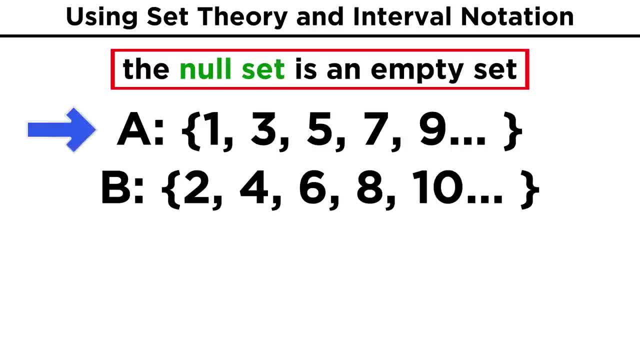 let's find the intersection between the set containing all the odd natural numbers and the set containing all the even natural numbers. Because these sets have no elements in common, their intersection has nothing in it. This will be the empty set, otherwise known as. 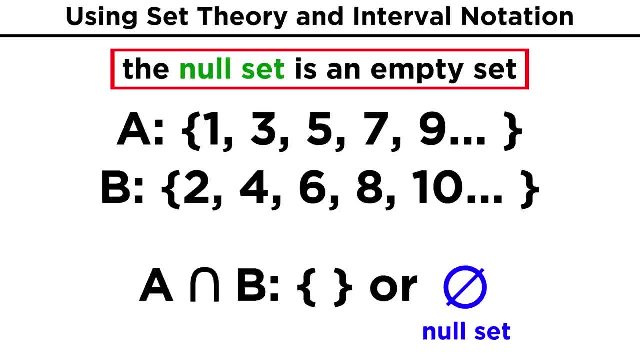 the null set. This is represented by the Greek letter phi, which looks kind of like a zero with a line through it. Remember, this isn't zero, because zero is an element that could be included in a set. The null set means there is nothing in it, not even zero. As we said, we can use.